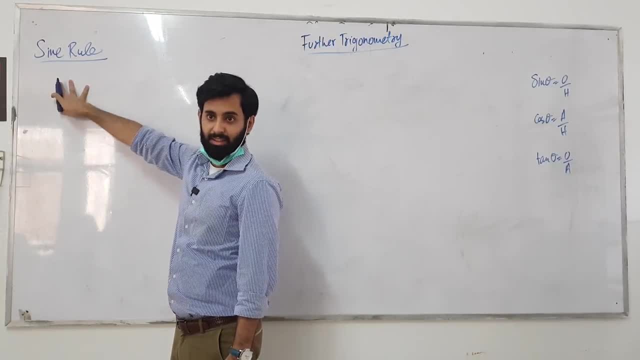 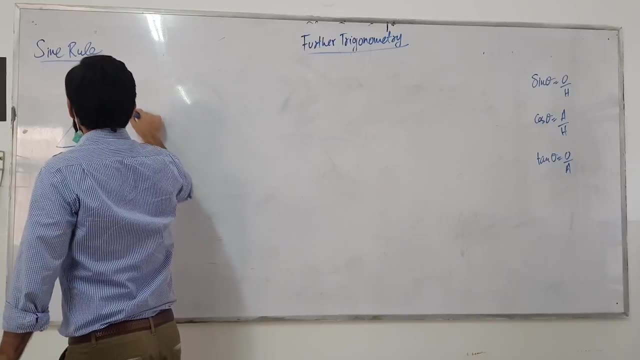 It is not that they cannot be applied in a 90 degree triangle, But we are going to use these because they are a lot easier to apply. First, you guys already know how to do it right. A, B, C. 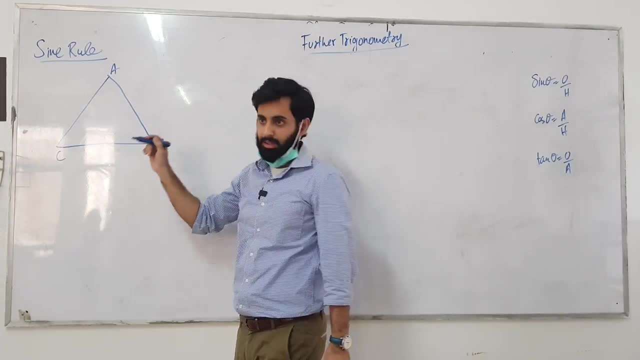 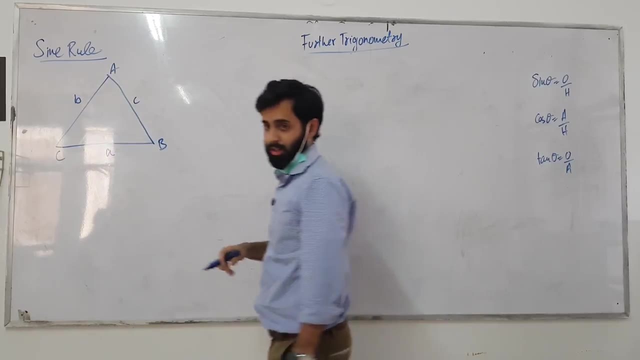 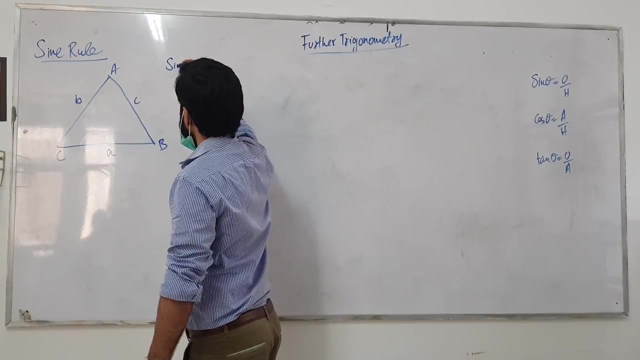 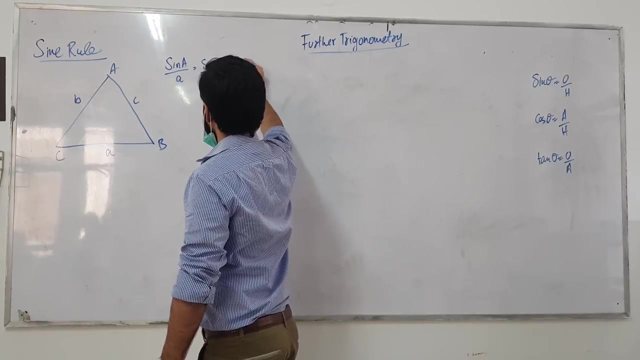 A. capital letters are used to represent angles. In case we are going to write lower case letters, and we are going to use them to represent lengths. Okay, Sorry. Now, first of all, let us see what the formula is. Sine A upon A equals to sine B upon B is equal to sine C upon C. 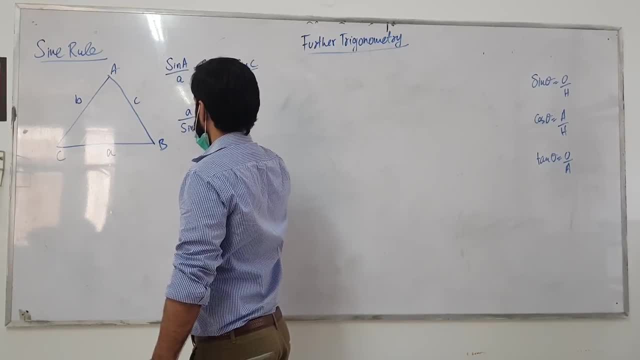 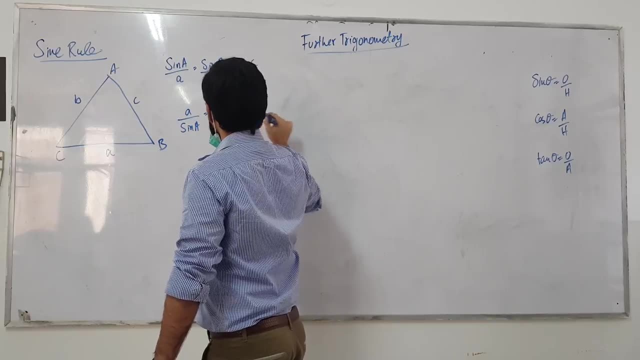 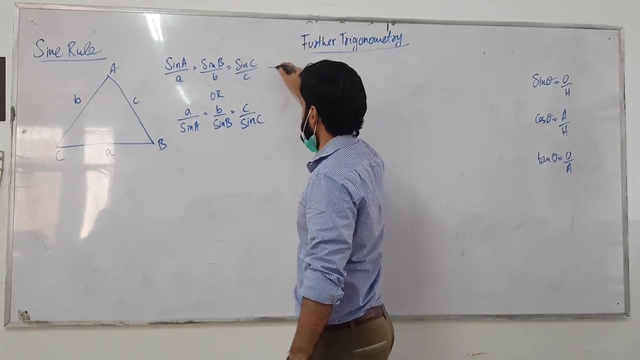 We can write them like this: It's same as before. Sorry, Same as before. Same as before. I will tell you guys when and if we are going to use it, Although you can use whichever form you want, Okay, But it is preferable to use this form when you need to find an angle. 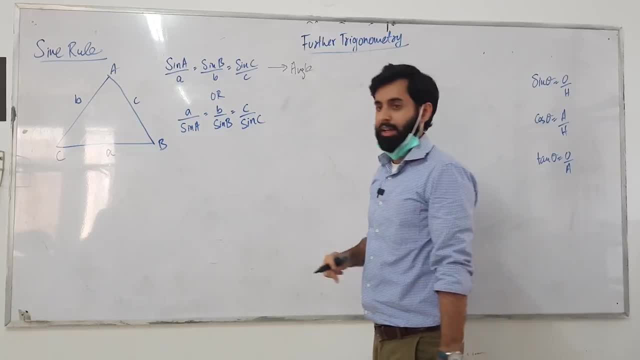 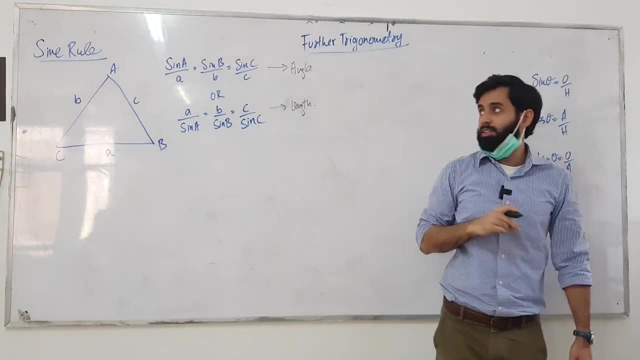 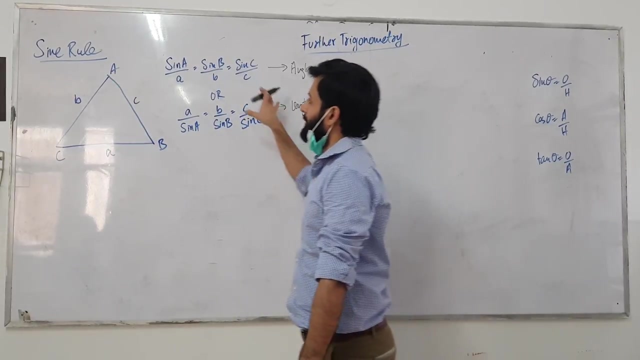 Okay, We are going to use this if you need to find an angle, And we are going to use this if we need to find any missing length. The idea here is to keep the unknown in the numerator, because that makes things a lot easier. I said that when our unknown is in the numerator, it becomes easy to calculate. 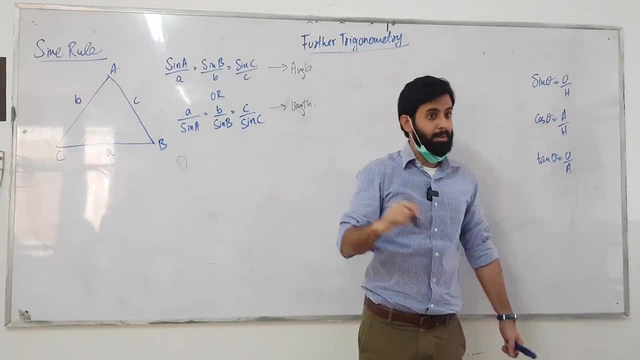 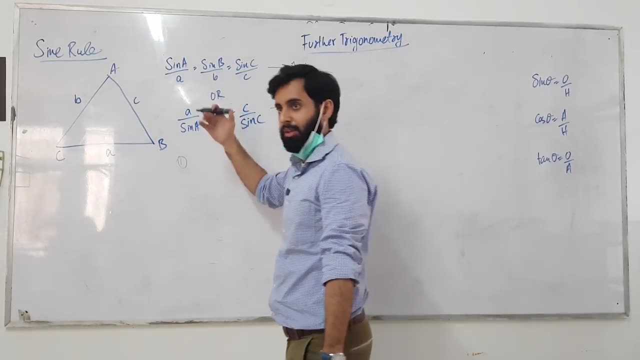 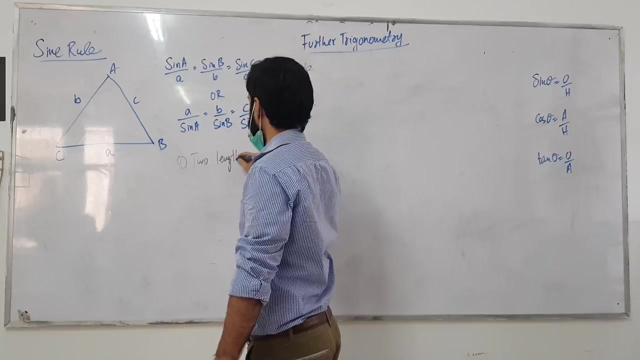 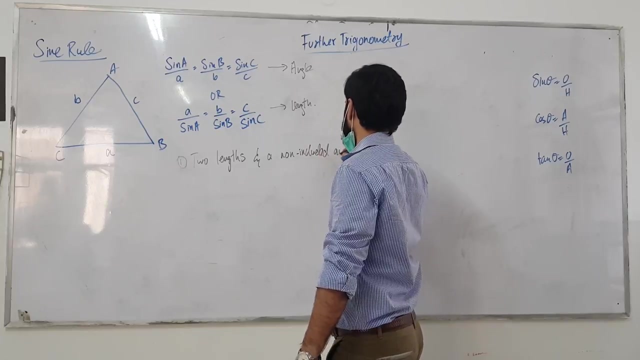 Alright, now this is the formula. Like the formula of the area of triangle, this is also the new formula. Now there are some conditions when we apply the formula. We apply this when you have two lengths and a non-included angle. You guys know what an included angle is, right? 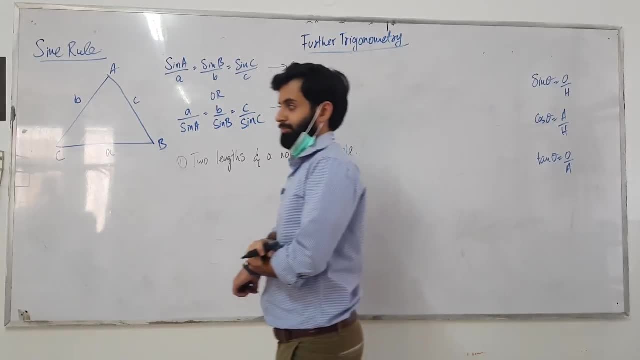 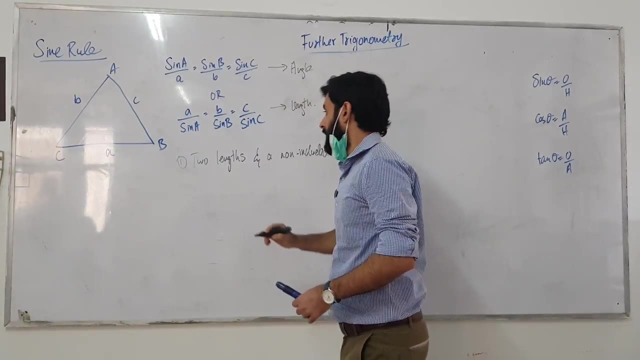 What happens to the non-included angle? I mean, what is an included angle? tell me, in between, Between two lengths. So what happens to the non-included angle? Anything other than the included angle, Or We use a new formula. 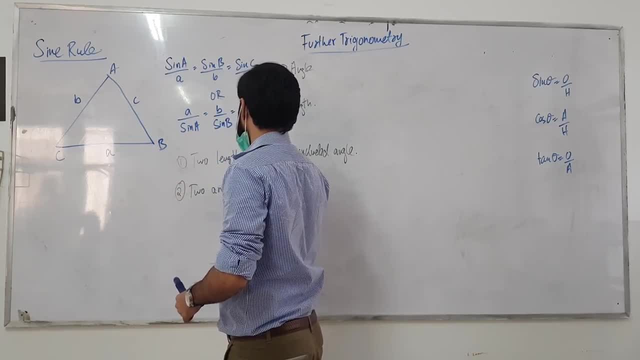 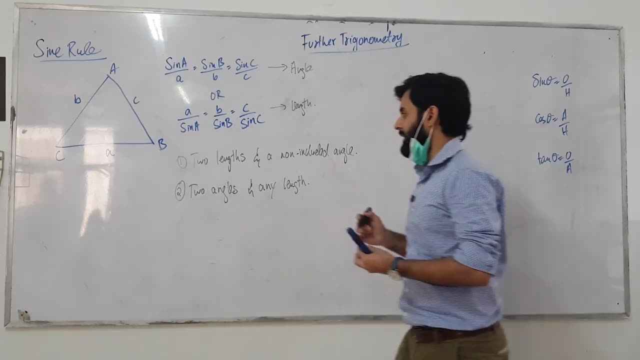 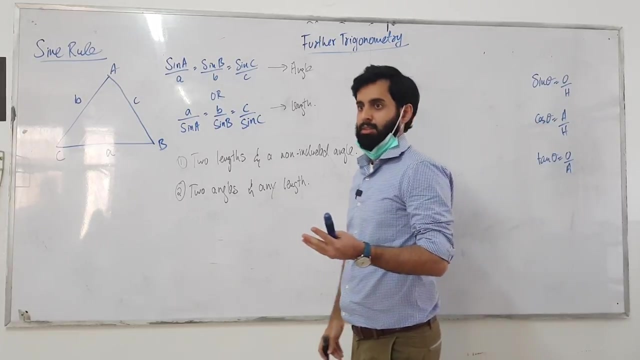 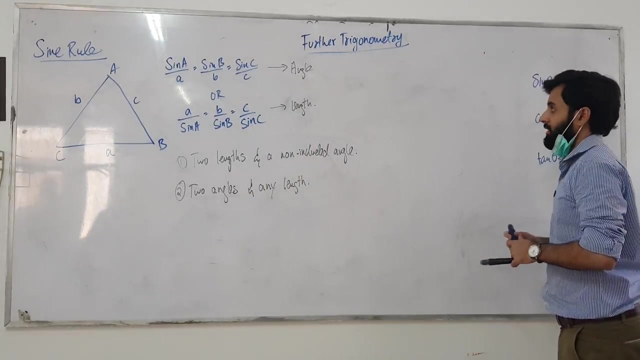 is, we have two angles and any length. If I give you two angles in a triangle, so does that mean you cannot figure out the third one? You can. you can take these two angles. you can sum them up and subtract it from 180 and figure out the third angle. you guys at. 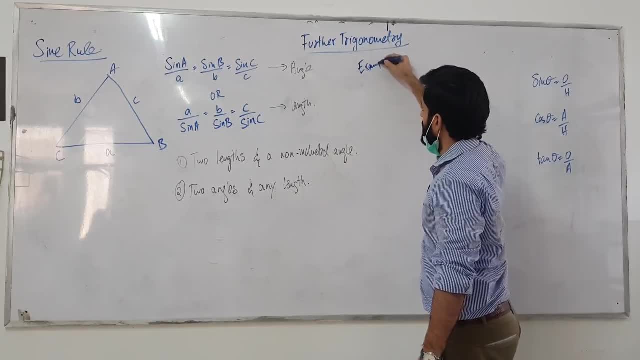 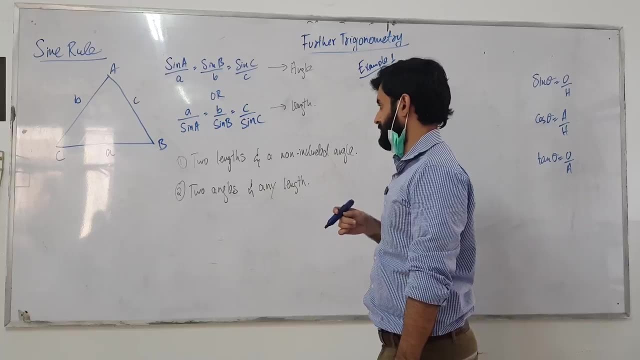 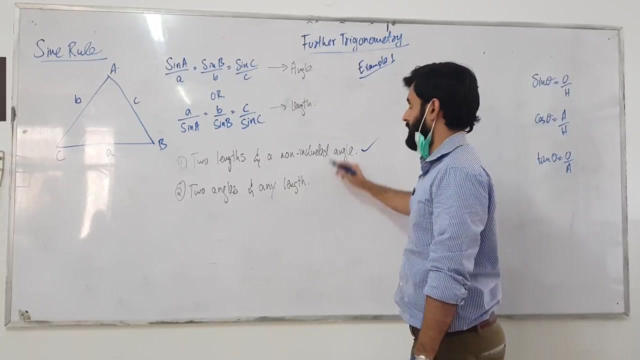 the back, pay attention. Okay, let's do an example. Yes, These are the two conditions, or we can apply it in this condition. yes, yes, look, we will apply this when we need an angle. Now, obviously, if we have two angles, that means we can figure. 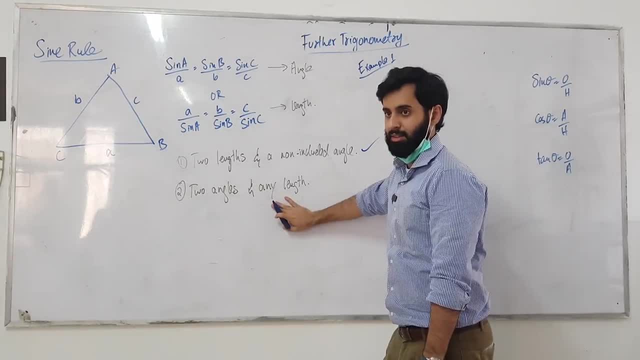 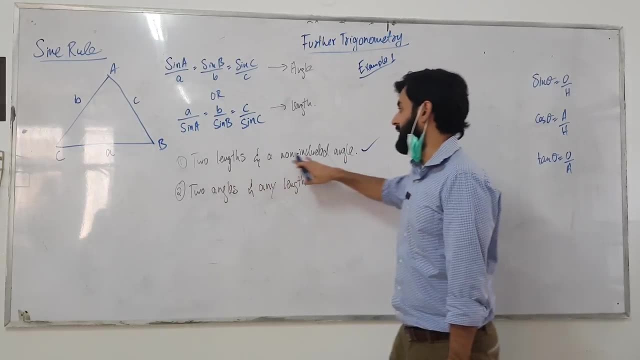 out the third angle. And what do you have? You have one length, let's say that means what is the question you are going to ask? Obviously, it will ask you to figure out any length. okay Here, if you have two lengths. 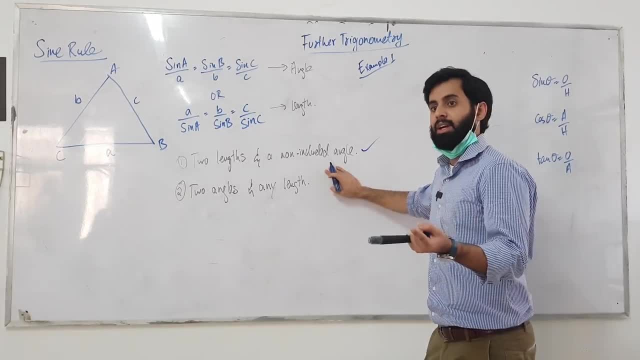 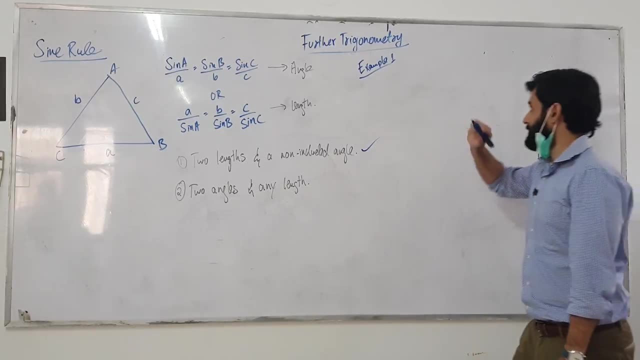 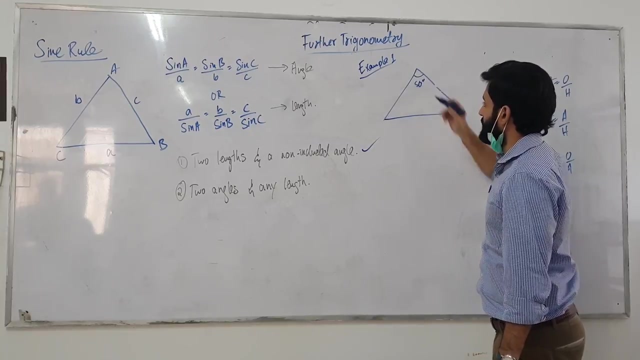 and one angle. so it can ask you one of the two, either to figure out the third length or any missing angle. This, Wait, now you will understand. just give me a minute. Okay, let's say this is 50 degrees in front of 50 degrees. I will give you 12 centimeters. 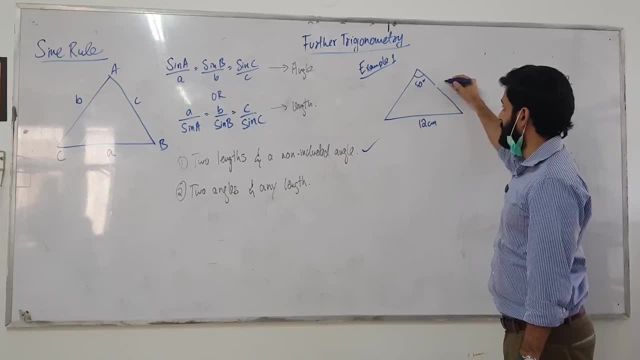 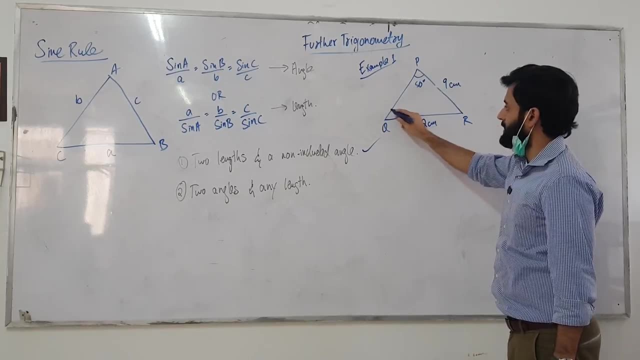 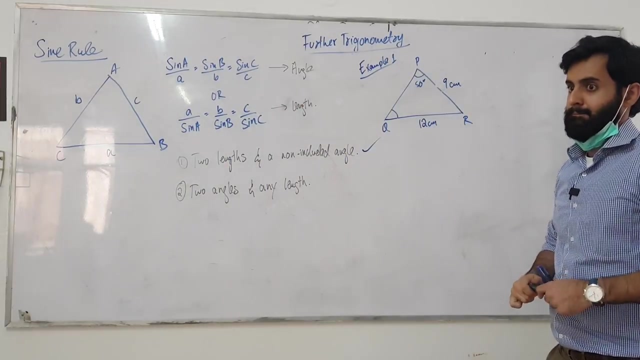 okay, Yes, Okay. So you can just give me the length, Okay, Okay, If I give you 12 centimeters, then this is to be 9 centimeters. Yes, Let's say. I ask you guys to figure out this angle. 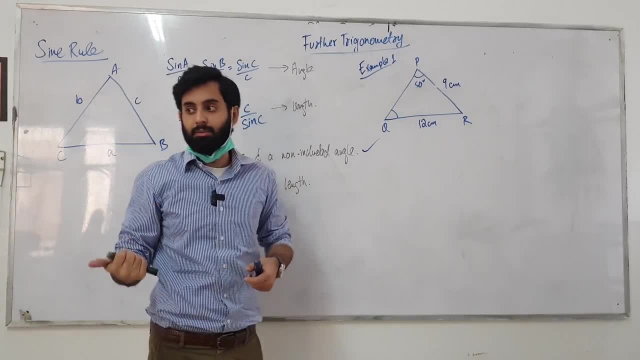 Sir, you can even just sign. then it is a right angle rather than triangle. We can apply this to any triangle. Look what is hypotenuse: It is in any triangle, or it is only in the right angle. It is in the right angle. 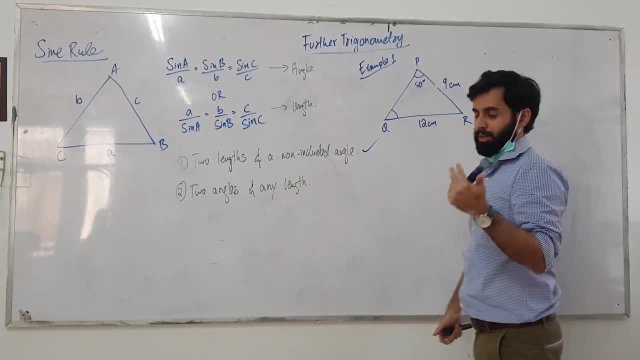 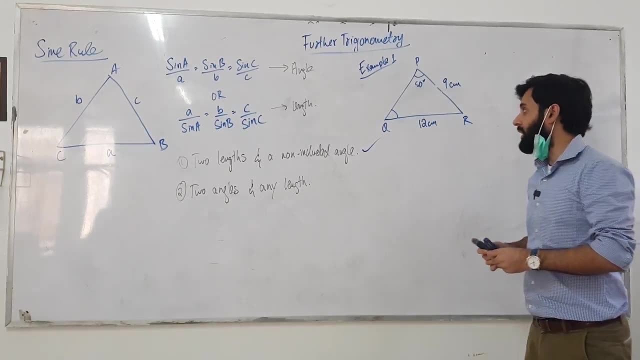 Only in the right angle. So what I have just erased, sign cost, and opposite upon hypotenuse, adjacent upon hypotenuse. which one can we apply? This one, Okay? Okay, Let's say we have to figure out angle Q. 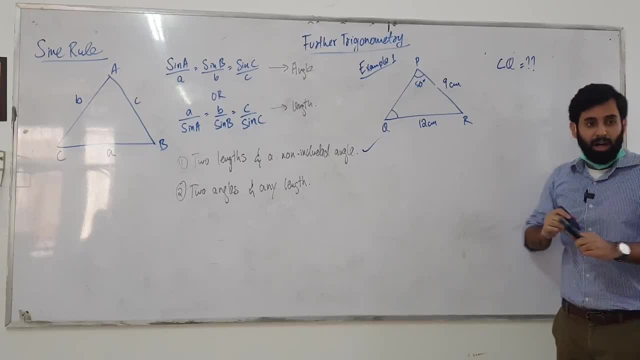 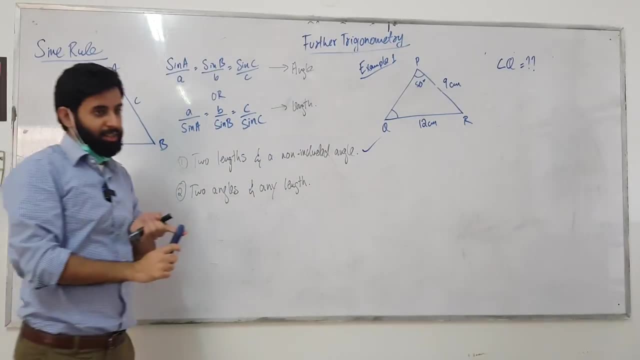 What do we have to find? We have to find angle Q. Now, before applying sine rule, one condition is that you should have a pair complete. What does a pair complete mean? You should have an angle and a length in front of it. 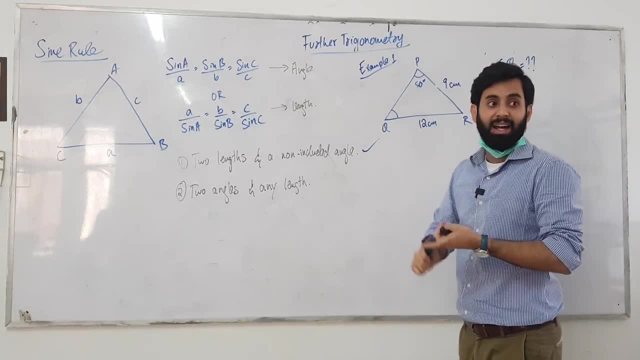 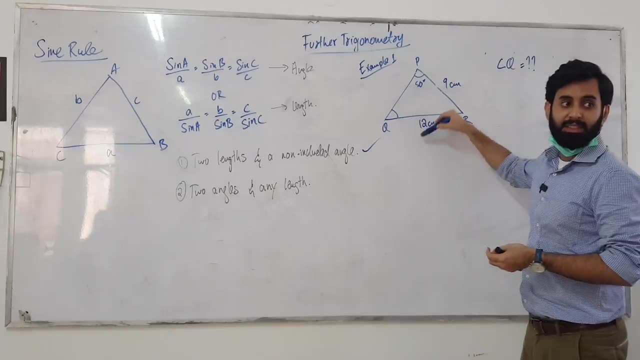 Or in other words, you should have a length and an angle in front of it. Look here carefully and tell me, is there a pair like this? Yes, It is being made. We have an angle and a length in front of it. 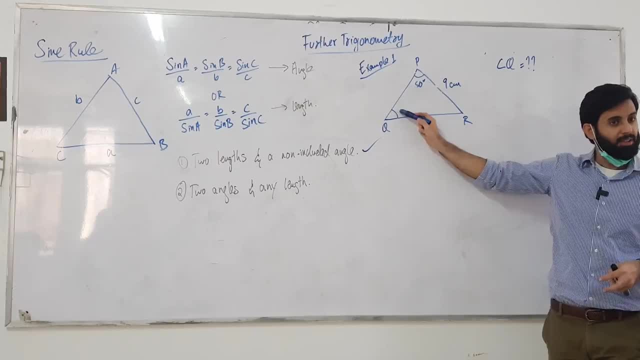 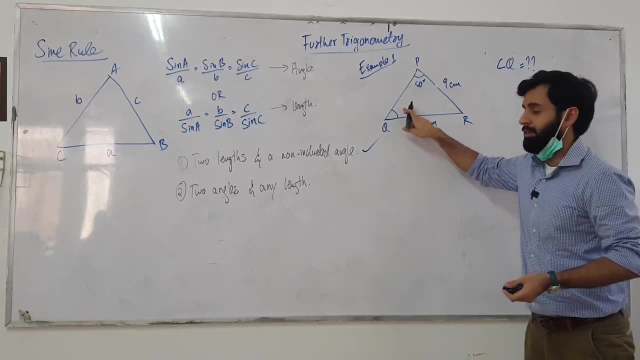 Now what is here? This pair is incomplete. Why is that? Because we have the length, but we don't have the angle. So this is how we will start. What do we have to find out? We have to find out angle Q. 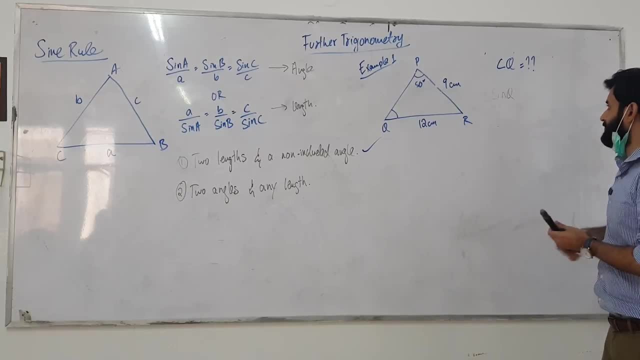 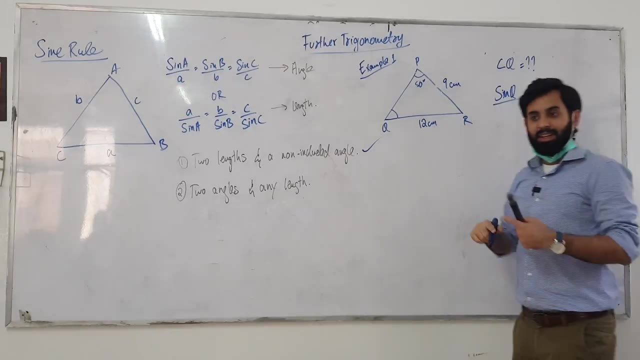 So, first of all, we will write sine Q, Not theta Q. Below this, we will write the length that is opposite of Q, Which is 9.. Which is 9.. Okay, Now, this ratio is going to be the same as. 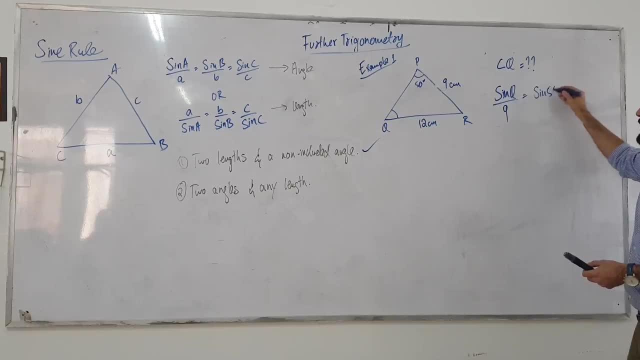 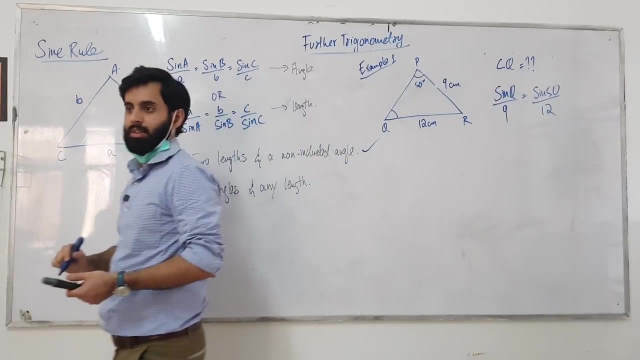 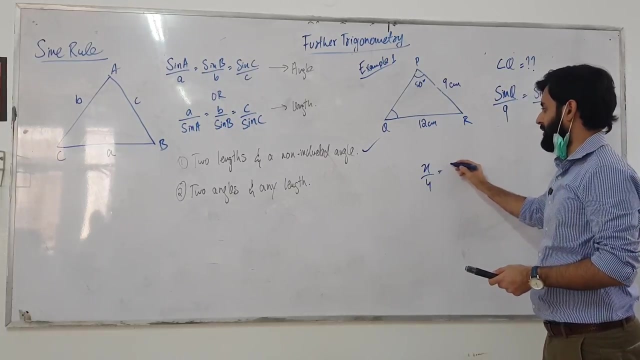 sine 50 upon 12.. Now pick up your calculators. This is not necessary, Because if you guys remember similar triangles, you might have understood this. X upon 4 equals to, let's say, 7 upon 14. 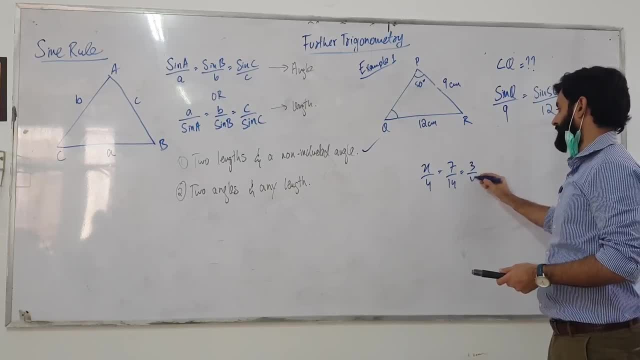 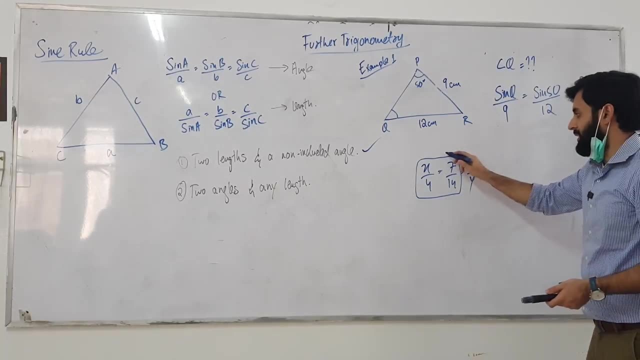 equals to, let's say, um 3 upon Y. Now, if we had to take out X, what would we do? We would use both of them. And if we had to take out Y, what would we do? We would use both of them. 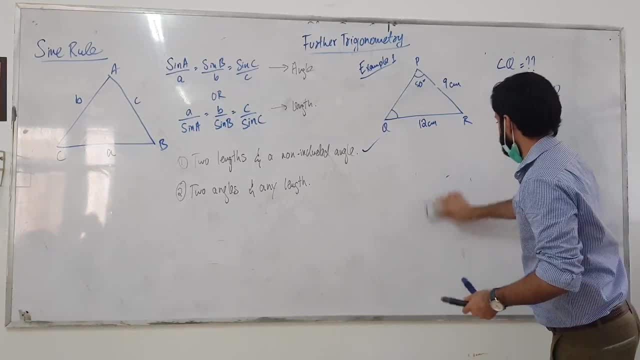 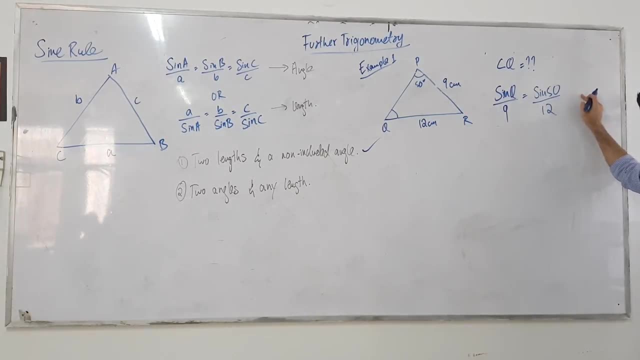 Okay, So that's the objective here also. Okay, Now here's what I want you guys to do: Write sine 50. Close the bracket. Divide it by 12.. Okay, yeah upon 12.. Press equals to. 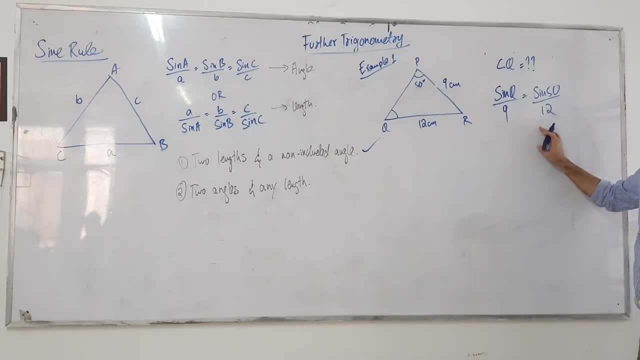 Inverse sine: Sabar, sabar, sabar, sabar. Okay, so you must have some value. What happens after 9?? It's going to get multiplied, Okay, So multiplied by 9.. Zero point five. 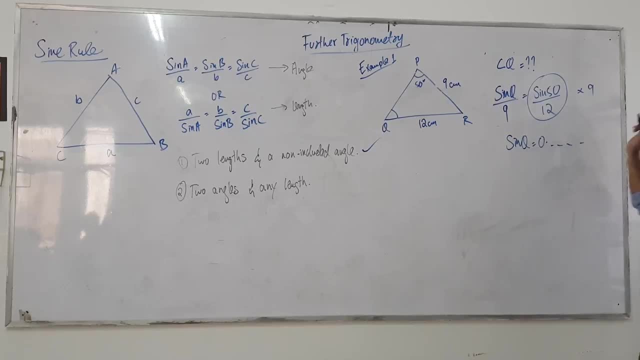 So this is where you are right now. Sine, Q equals to zero, point some value in your calculator. Now, if you want to find Q, what will you do? Sine, You're going to bring sine on the other side. 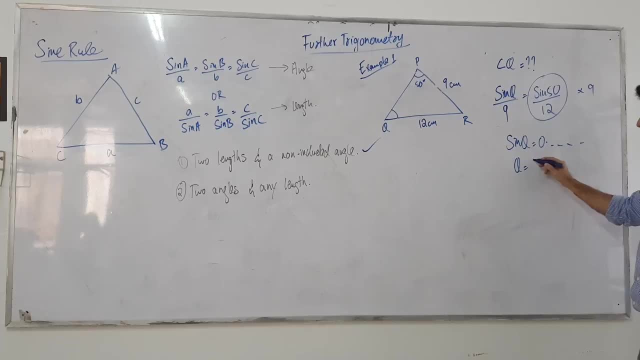 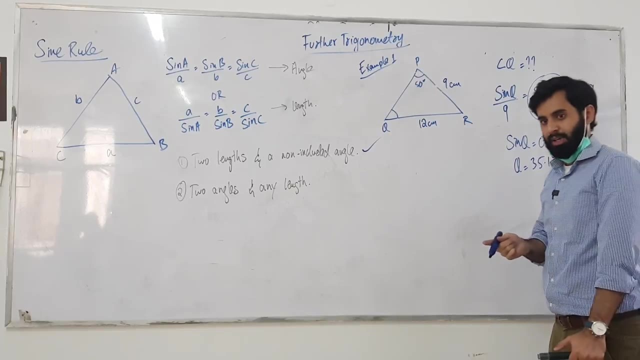 So it will become inverse, So sine inverse, of your answer And you're going to get what You're going to get: 35.1.. Okay, you've got to remember that angles are always given correct to one decimal place. 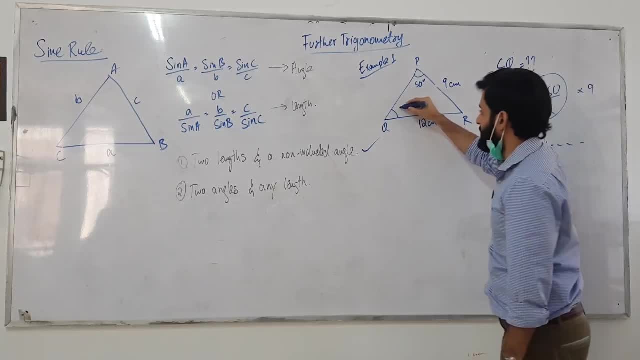 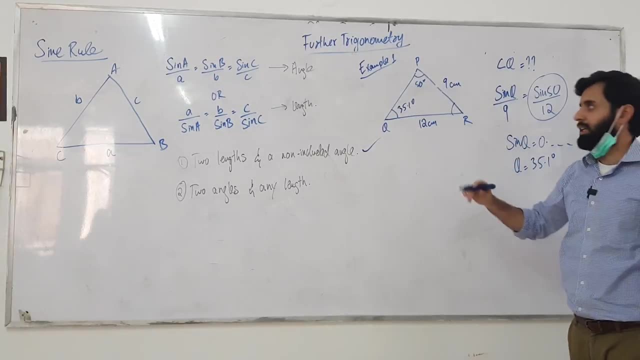 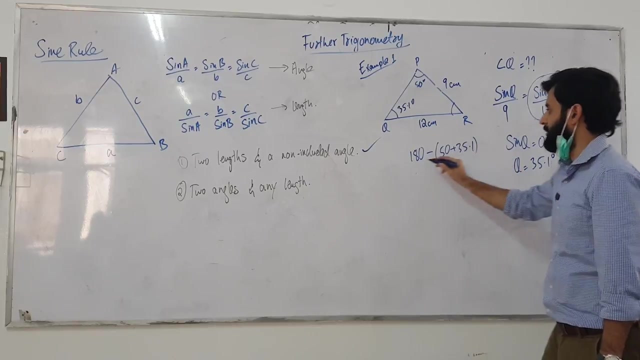 Okay, Angles are given correct to one decimal place. So that means we have successfully figured out angle Q. Now tell me, can we find angle R Without using sine rule? Absolutely, How will we find it? 180 minus 50 plus 35.1.. 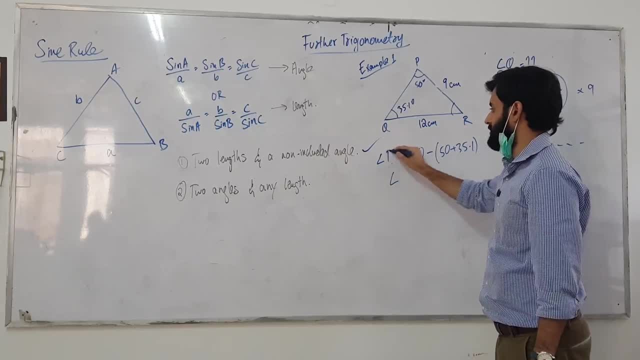 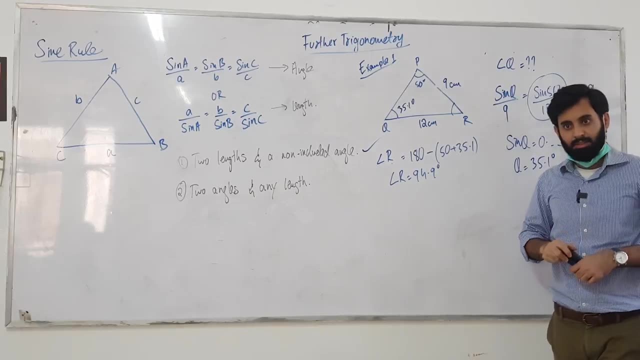 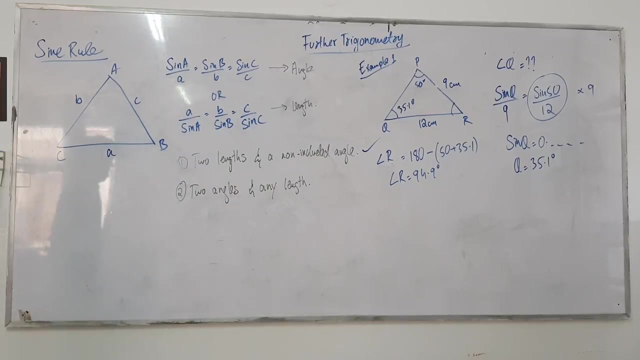 So this is our angle Q, Sorry, angle R. Angle R equals to 94 point Nine degrees. Any questions Difficult to keep up with. We'll do more examples. Copy it quickly. We'll do more examples. Angle is opposite to length. 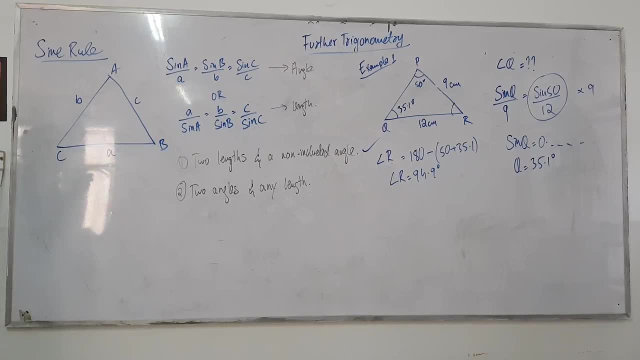 Like, if angle is same, so the length that's opposite to it is length. Yeah, Just say capital C. the length that's opposite to it is lowercase c. Capital B: the length that's opposite to it is lowercase b. 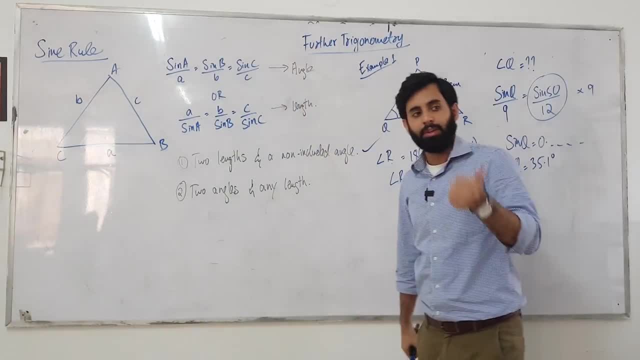 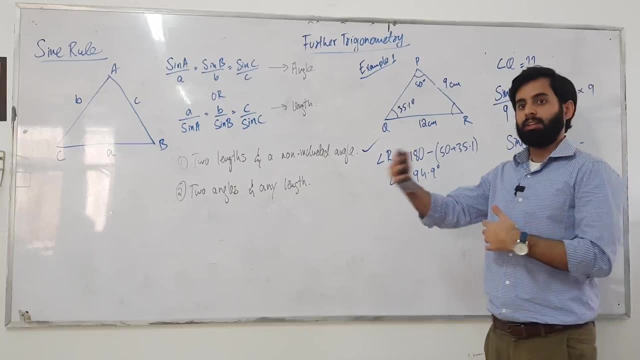 Okay. So basically, long story short. you guys should remember this: Before you can apply sine rule, you should have a pair, Okay, And that pair should consist of an angle and the length opposite to that angle. Only then you'll have a fraction. 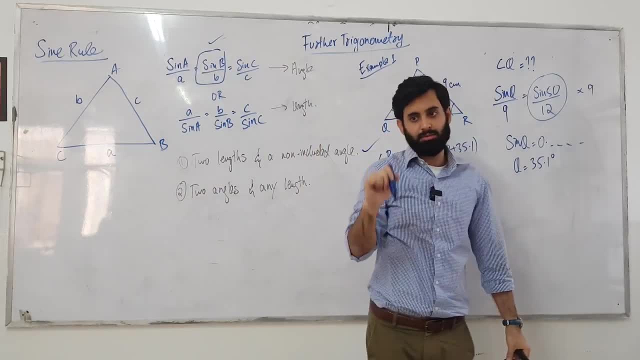 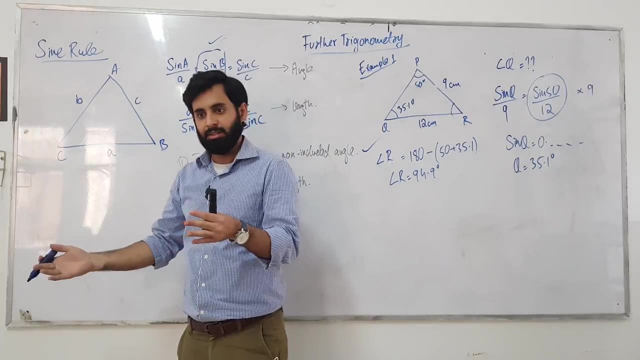 whose numerator and denominator you'll know. Okay, Yes, Then if you have an angle that doesn't have the length in front of it, then you can remove it. Or in other words, if you have the length but you don't have an angle, 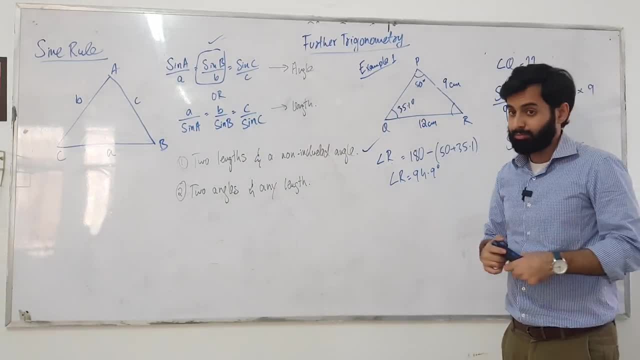 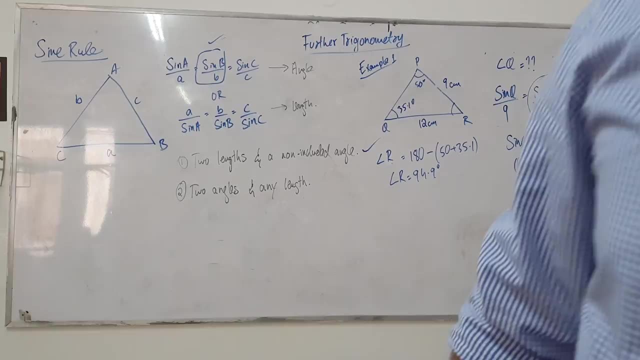 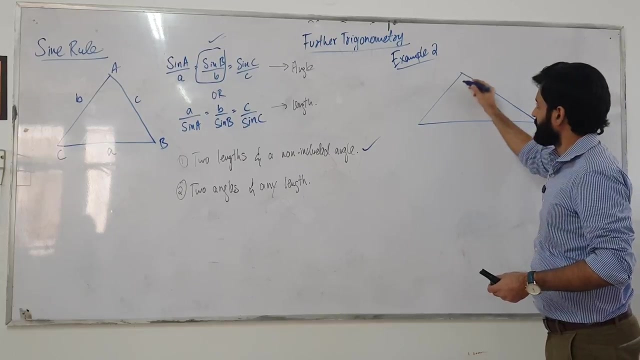 then you can remove it. You need to know what's not certified. Sorry, You need to know what's not certified. Yeah, Can you copy this? Are you still rolling? All right? So here's the next example. Let's quickly do this and wind it up. 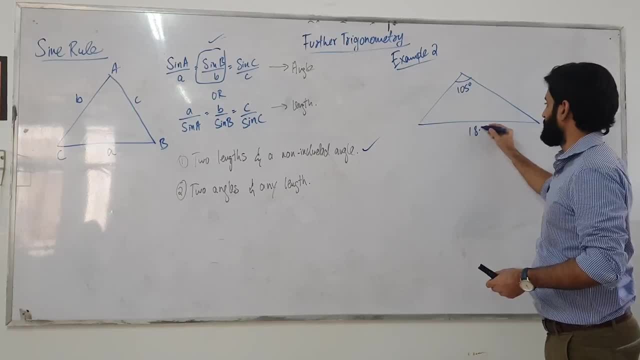 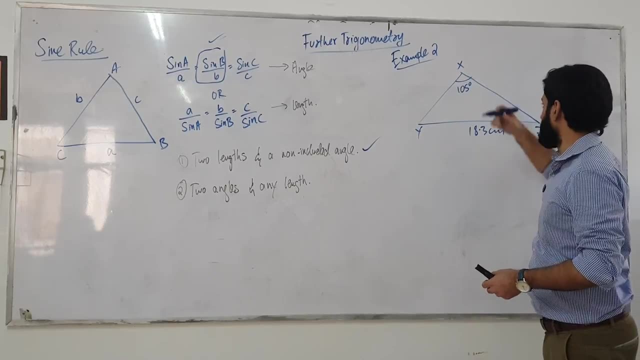 Okay, Let's say here's one of five degrees. Okay, Let's say here's 18.3 centimeter. Let's say this is x, y, z. Okay, Now you are given this length: 11 centimeter. 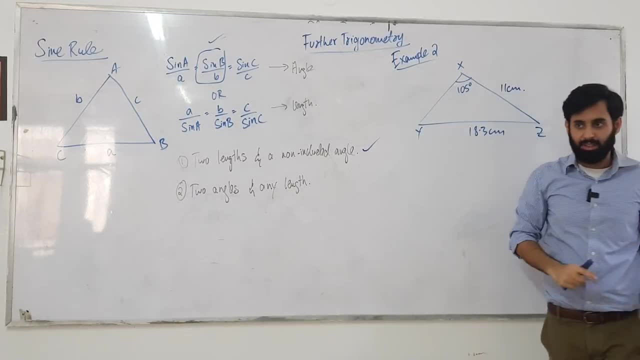 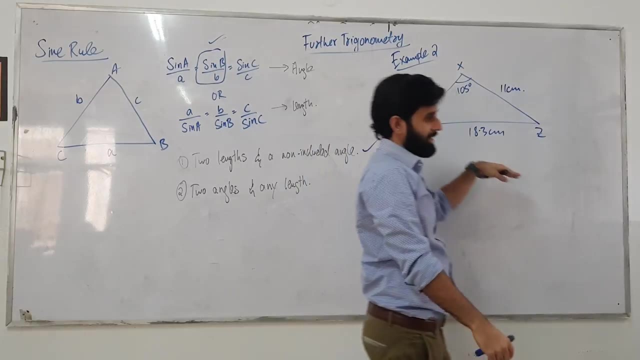 Okay, First, have a look at this triangle. Have a good look at this triangle And tell me: can we apply the sine rule on this or not? Yes, you can. You can Why? Because one of our pairs is complete. 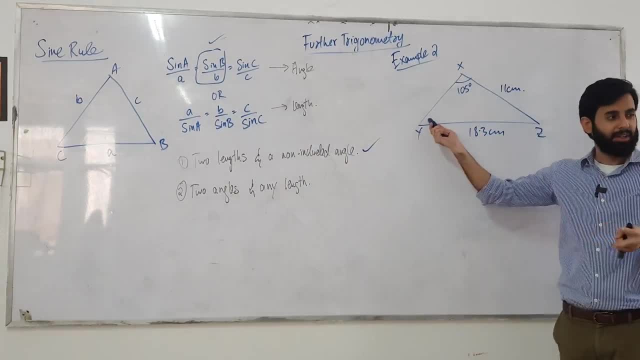 We have the angle and the length opposite to it. This pair is incomplete because we don't have what Angle. We don't have the angle. However, we still have the length. Okay, So how are we going to start? This is how we'll start. 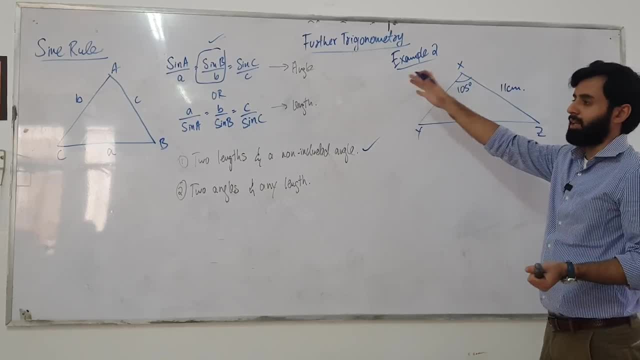 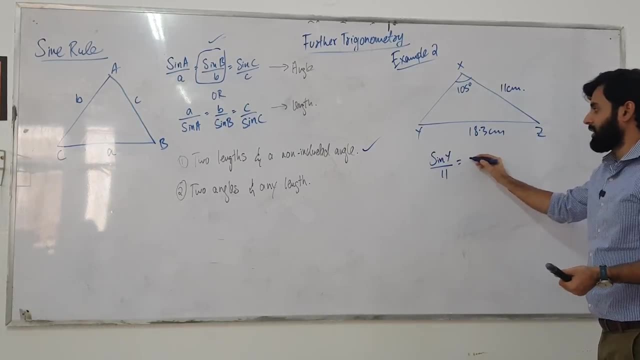 Sine a, Sine y. Now see this: a, b, c doesn't mean that the triangle will always be a, b, c, a. okay, So sine y upon 11 equals to sine 105.. X, which is 105, you're right upon 18.3.. 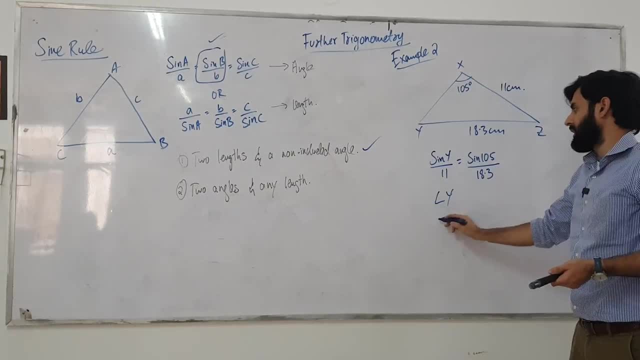 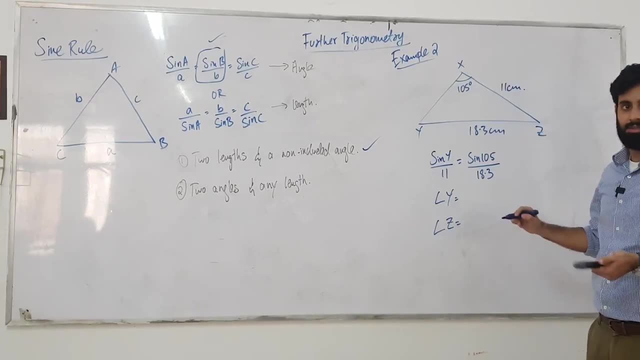 Okay, Now pick up your calculators quickly. Quickly give me the angle y and quickly give me the angle z. The answer is 34.5.. Does everyone agree with Suhaima? No, the angle y is 35.5..